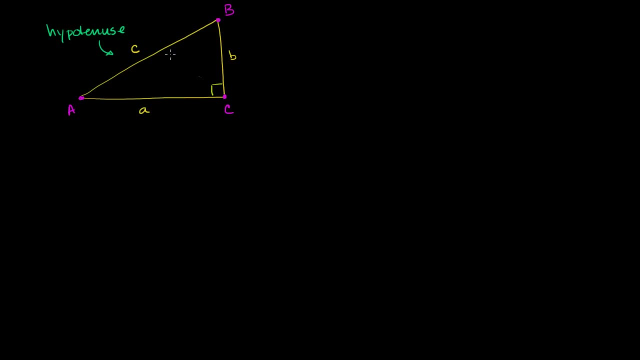 And let's see if we can come up with a relationship between A, B and C. And to do that, I'm first going to construct another line or another segment, I should say between C and the hypotenuse, and I'm going to construct it. 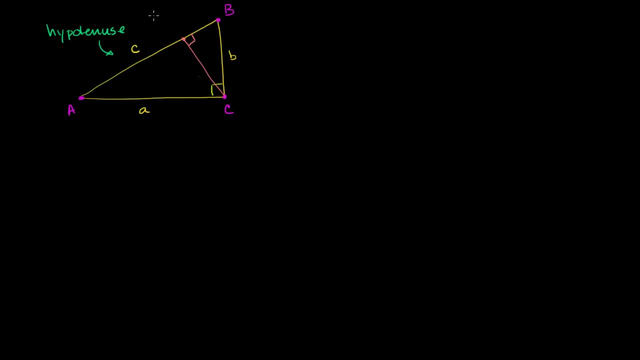 so that they intersect at a right angle. And you can always do that and we'll call this point right over here, we'll call this point capital D And if you're wondering how can you always do that, You can imagine rotating this entire triangle like this: 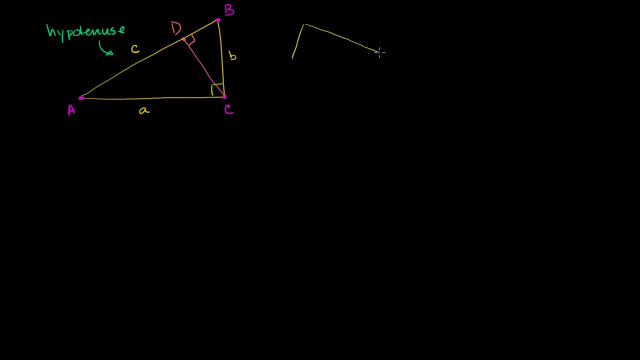 and this isn't a rigorous proof, but it just kind of gives you the general idea of how you can always construct a point like this. So, if I've rotated it around, so now our hypotenuse. we're now sitting on our hypotenuse. 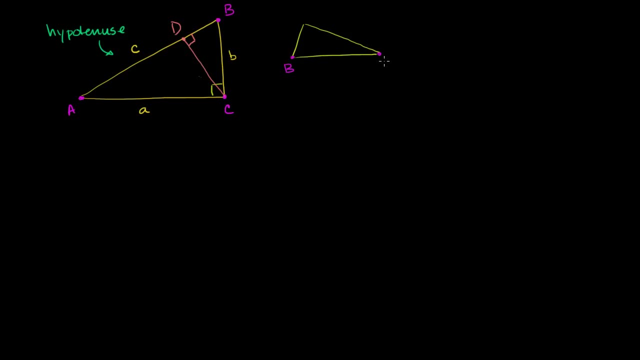 This is now point B. this is point A, So we've rotated the whole thing all the way around. This is point C. You can imagine just dropping a rock from point C, maybe with a string attached, and it would hit the hypotenuse at a right angle. 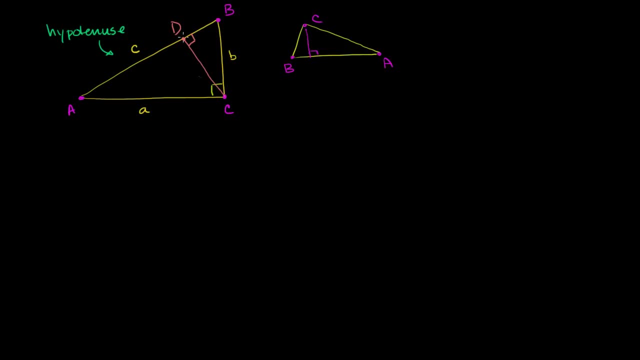 So that's all we did here to establish segment CD into where we put our point D right over there. And the reason why I did that is now we can do all sorts of interesting relationships between similar triangles, because we have three triangles here: We have triangle ADC, we have triangle DBC. 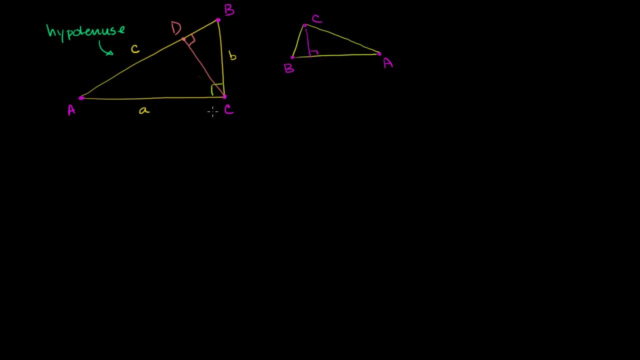 and then we have the larger original triangle And we can hopefully establish similarity between those triangles. And first I'll show you that ADC is similar to the larger one because both of them have a right end and ADC has a right angle right over here. 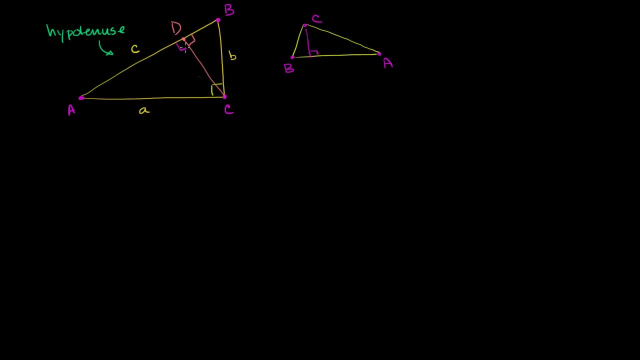 Clearly, if this angle is 90 degrees, then this angle is going to be 90 degrees as well. They're supplementary, They have to add up to 180. And so they both have a right angle in them. So the smaller one has a right angle. 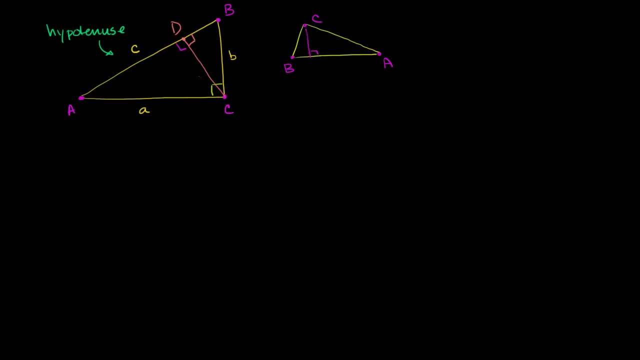 The larger one clearly has a right angle. That's where we started from And they also both share this angle right over here, angle DAC or BAC, however you want to refer to it, So we can actually write down that triangle. I'm going to start with the smaller one. 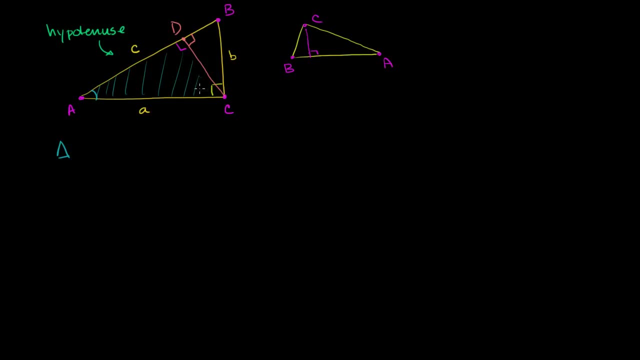 ADC and maybe I'll shade it in right over here. So this is the triangle. we're talking about triangle ADC, And I went from the blue angle to the right angle to the unlabeled angle, from the point of view of triangle ADC. 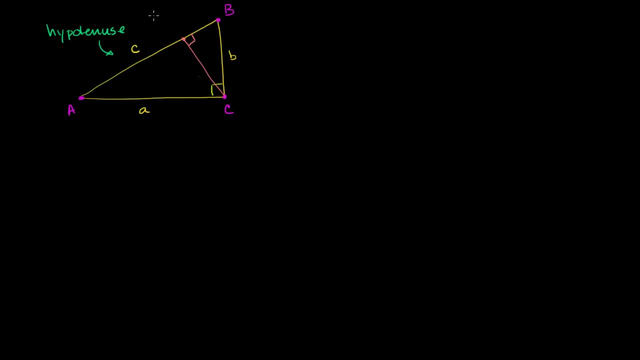 so that they intersect at a right angle. And you can always do that and we'll call this point right over here, we'll call this point capital D And if you're wondering how can you always do that, You can imagine rotating this entire triangle like this: 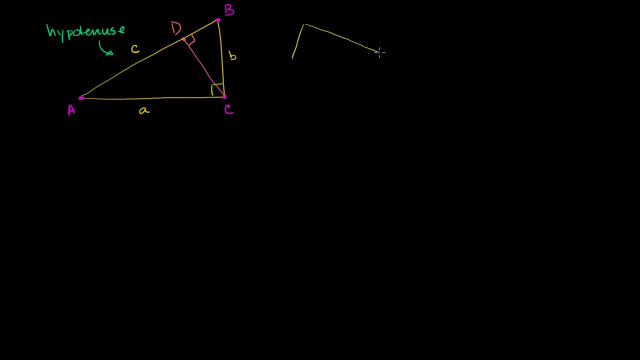 and this isn't a rigorous proof, but it just kind of gives you the general idea of how you can always construct a point like this. So, if I've rotated it around, so now our hypotenuse. we're now sitting on our hypotenuse. 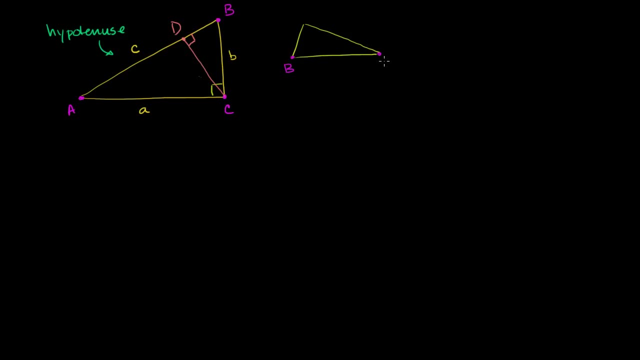 This is now point B. this is point A, So we've rotated the whole thing all the way around. This is point C. You can imagine just dropping a rock from point C, maybe with a string attached, and it would hit the hypotenuse at a right angle. 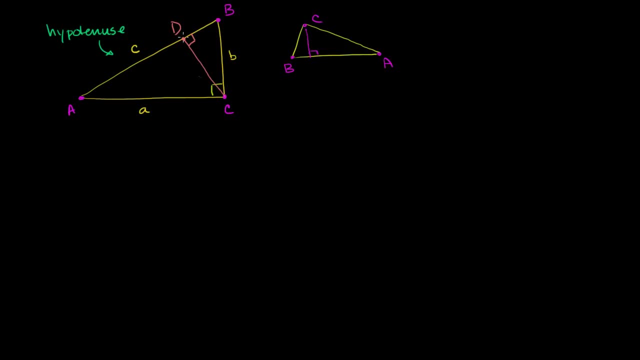 So that's all we did here to establish segment CD into where we put our point D right over there. And the reason why I did that is now we can do all sorts of interesting relationships between similar triangles, because we have three triangles here: We have triangle ADC, we have triangle DBC. 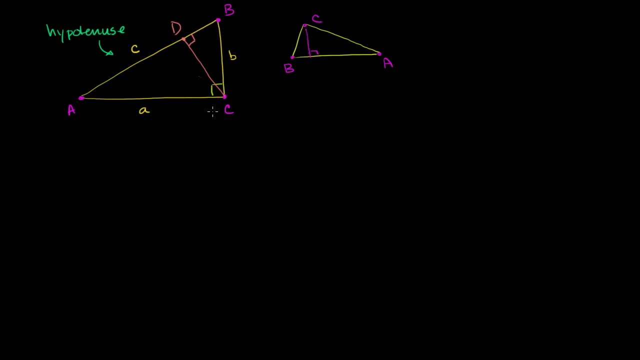 and then we have the larger original triangle And we can hopefully establish similarity between those triangles. And first I'll show you that ADC is similar to the larger one because both of them have a right end. ADC has a right angle right over here. 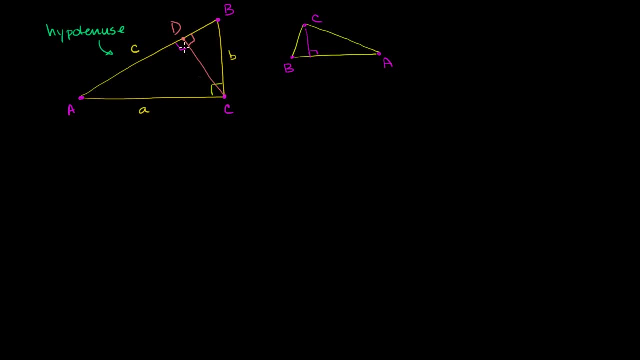 Clearly, if this angle is 90 degrees, then this angle is going to be 90 degrees as well. They're supplementary, They have to add up to 180. And so they both have a right angle in them. So the smaller one has a right angle. 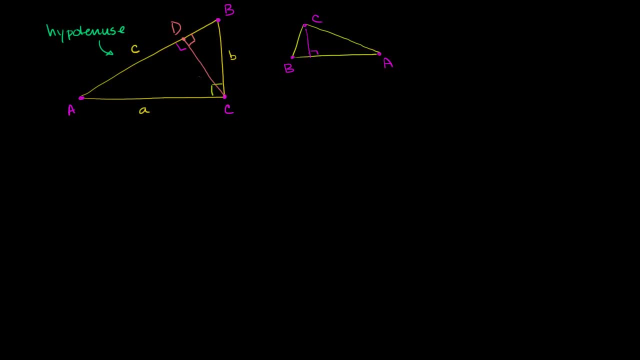 The larger one clearly has a right angle. That's where we started from And they also both share this angle right over here, Angle DAC or BAC, however you want to refer to it, So we can actually write down that triangle. I'm going to start with the smaller one. 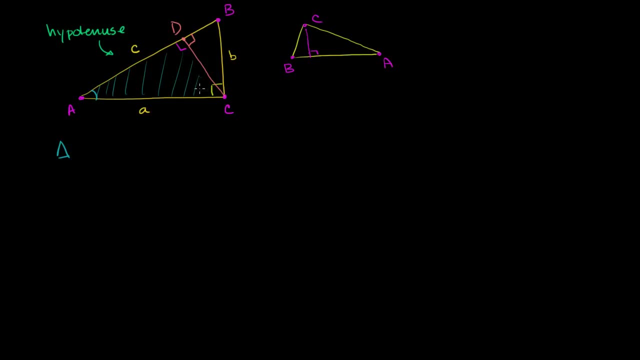 ADC and maybe I'll shade it in right over here. So this is the triangle. we're talking about Triangle ADC, and I went from the blue angle to the right angle to the unlabeled angle from the point of view of triangle ADC. 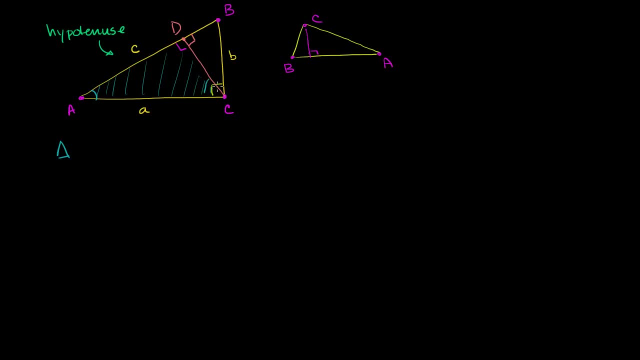 This right angle isn't applying to that right over there. It's applying to the larger triangle. So we can say triangle ADC is similar to triangle. Once again, you want to start at the blue angle A. Then we went to the right angle. 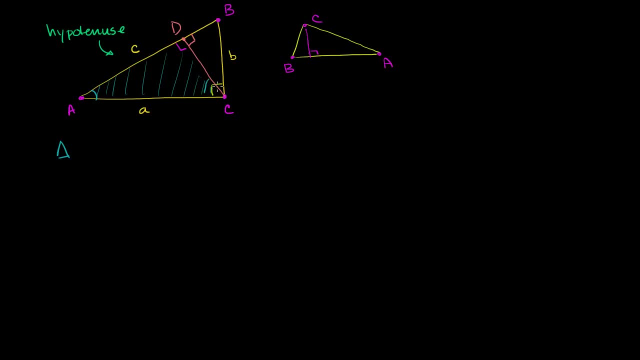 This right angle isn't applying to that right over there. It's applying to the larger triangle. So we can say triangle ADC is similar to triangle. Once again, you want to start at the blue angle A. Then we went to the right angle. 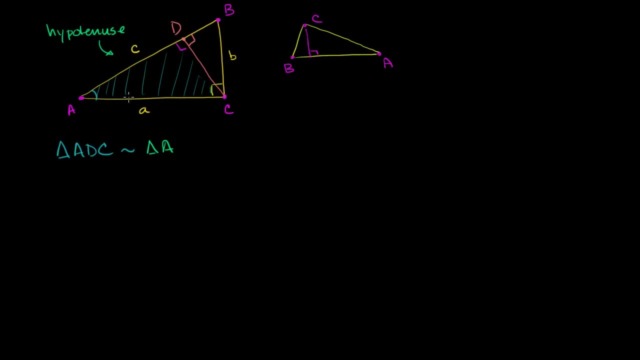 So we want to go to the right angle. again to triangle, so it's ACB And because they're similar we can set up a relationship between the ratios of their sides. For example, we know the ratio of corresponding sides are going to well in general for a similar triangle. 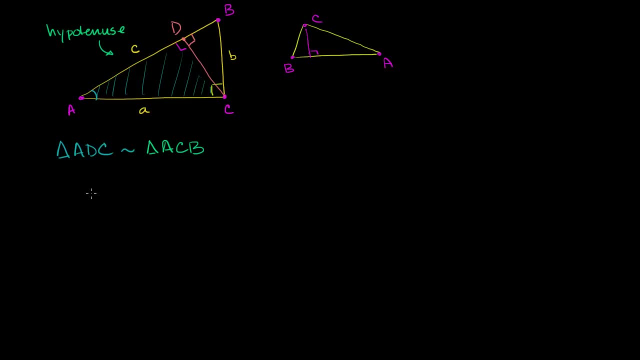 we know that the ratio of the corresponding sides are going to be a constant. So we could take the ratio of the hypotenuse of this side of the smaller triangle, So the hypotenuse is AC, Or the hypotenuse over the larger one, which is AB. 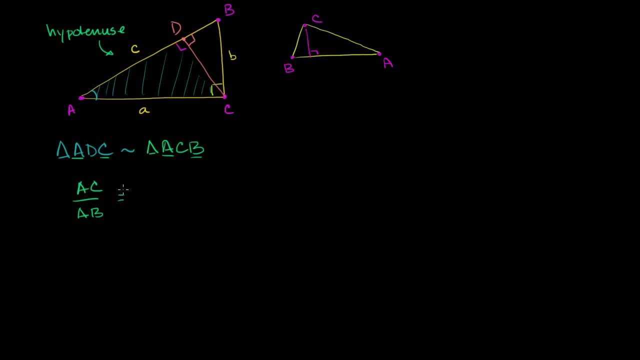 AC over AB is going to be the same thing as AD, as one of the legs AD. just to show that, I'm just taking corresponding points on both similar triangles. This is AD over AC. You could look at these triangles yourself and show. 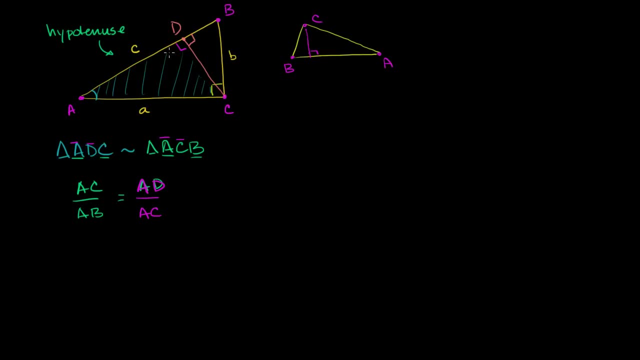 look AD point. AD is between AD and AD, AD over AC, AD over AC, AD over AC Side. AD is between the blue angle and the right angle Side. AC is between the blue angle and the right angle on the larger triangle. 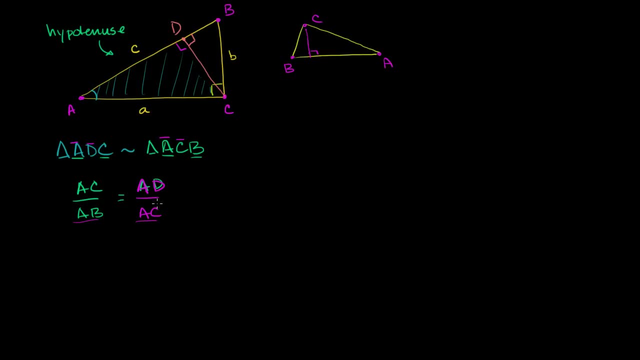 So both of these are from the larger triangle. These are the corresponding sides on the smaller triangle And if that is confusing looking at them visually, as long as we wrote our similarity statement correctly, you can just find the corresponding points. AC corresponds to AB on the larger triangle. 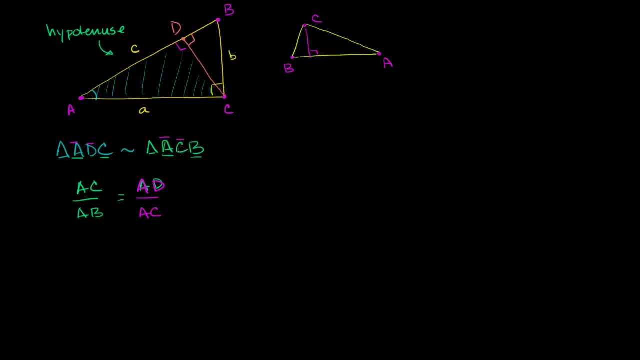 AD on the smaller triangle corresponds to AC on the larger triangle And we know that AC. we can rewrite that as lowercase a. AC is lowercase a. We don't have any label for AD or for AB. Sorry, we do have a label for AB. 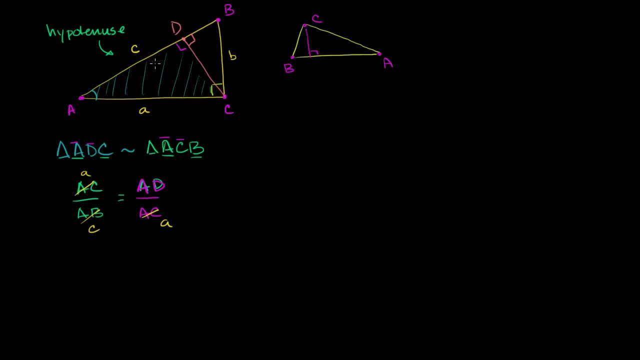 That is C right over here We don't have a label for AD, So let's just call that lowercase d. So lowercase d applies to AD, So that part right over there C applies to that entire part right over there, And then we'll call db. let's call that length e. 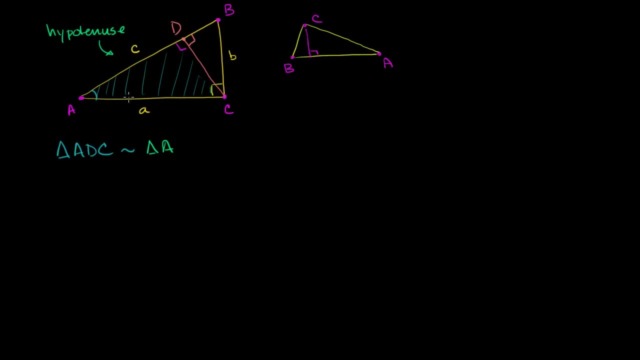 So we want to go to the right angle. again to triangle, so it's ACB And because they're similar we can set up a relationship between the ratios of their sides. For example, we know the ratio of corresponding sides are going to well in general for a similar triangle. 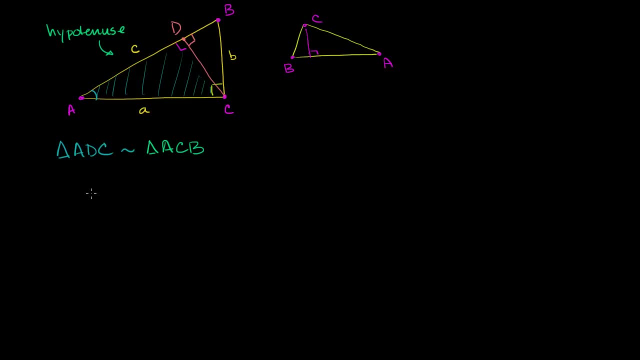 we know that the ratio of the corresponding sides are going to be a constant. So we could take the ratio of the hypotenuse of this side of the smaller triangle, So the hypotenuse is AC, Or the hypotenuse over the larger one, which is AB. 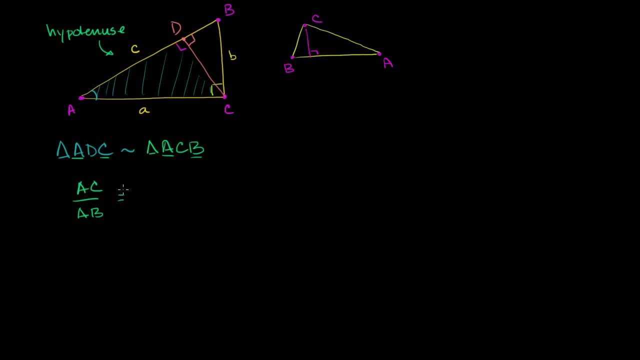 AC over AB is going to be the same thing as AD as one of the legs AD. Just to show that, I'm just taking corresponding points on both similar triangles. this is AD over AC. You could look at these triangles yourself and show. 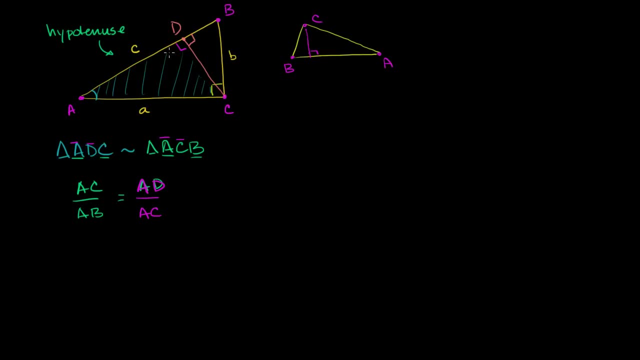 look AD point. AD is between AD and AD, AD over AC, AD over AC, AD over AC Side. AD is between the blue angle and the right angle Side. AC is between the blue angle and the right angle on the larger triangle. 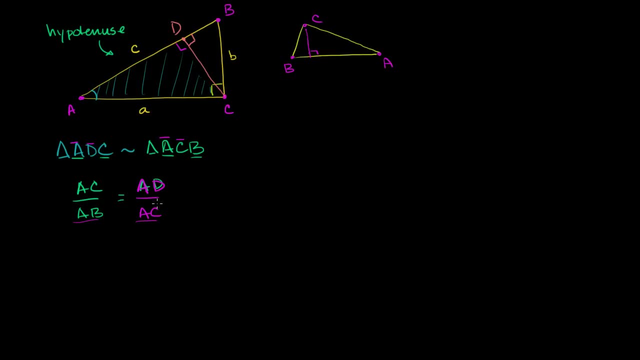 So both of these are from the larger triangle. These are the corresponding sides on the smaller triangle And if that is confusing looking at them visually, as long as we wrote our similarity statement correctly, you can just find the corresponding points. AC corresponds to AB on the larger triangle. 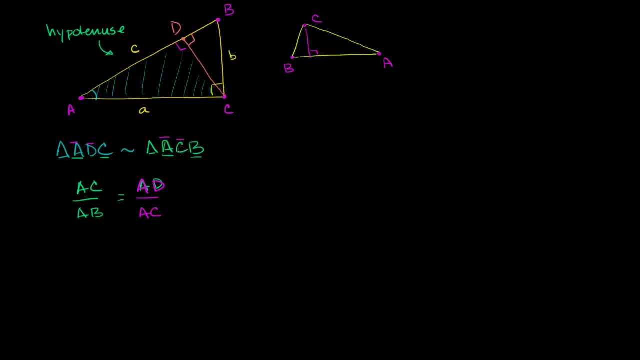 AD on the smaller triangle corresponds to AC on the larger triangle And we know that AC. we can rewrite that as lowercase a. AC is lowercase a. We don't have any label for AD or for AB. Sorry, we do have a label for AB. 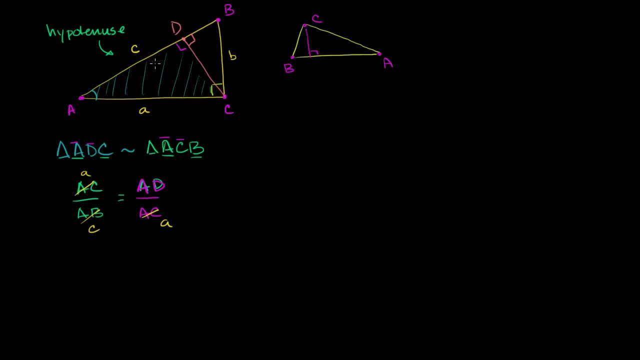 That is C right over here We don't have a label for AD, So let's just call that lowercase d. So lowercase d applies to AD, So that part right over there C applies to that entire part right over there, And then we'll call db. let's call that length e. 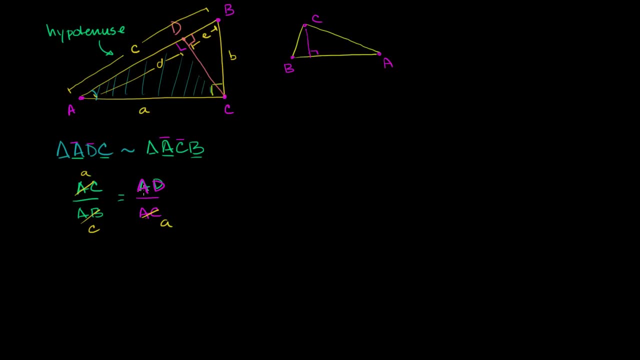 That'll just make things a little bit simpler for us. So AD we'll just call d, And so we have a over c is equal to d over a. If we cross multiply, you have a times a, which is a squared is equal to c, times d, which is cd. 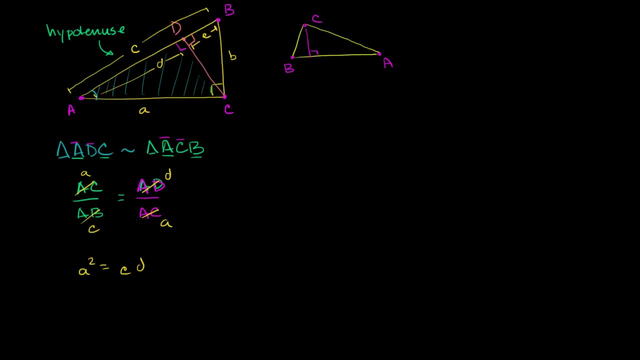 So that's a little bit of an interesting result. Let's see what we can do with the other triangle right over here. So this triangle right over here, So once again it has a right angle. The larger one has a right angle. 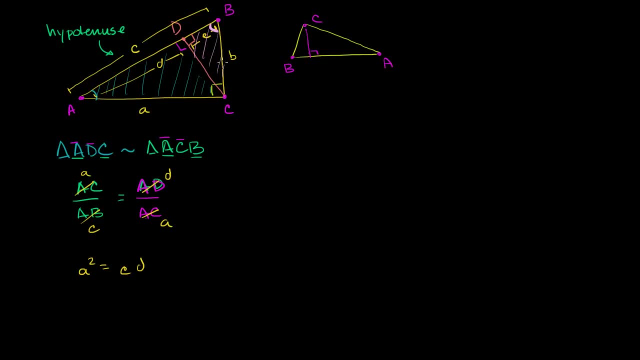 And they both share this angle right over here. So by angle-angle similarity the two triangles are going to be similar. So we could say triangle BDC. We went from pink to right to not labeled, So triangle BDC is similar to triangle. 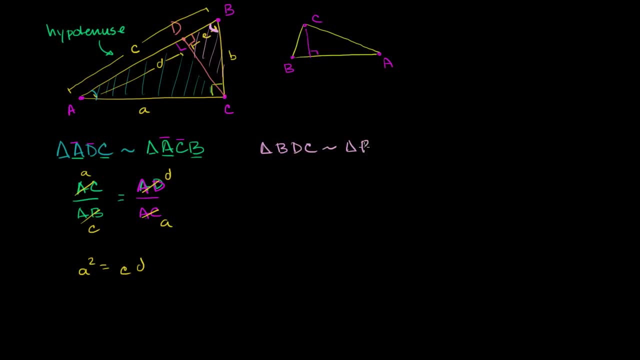 Now we're going to look at the larger triangle. We're going to start at the pink angle b Now. then we go to the right angle ca, From pink angle to right angle to non-labeled angle, at least from the point of view here. 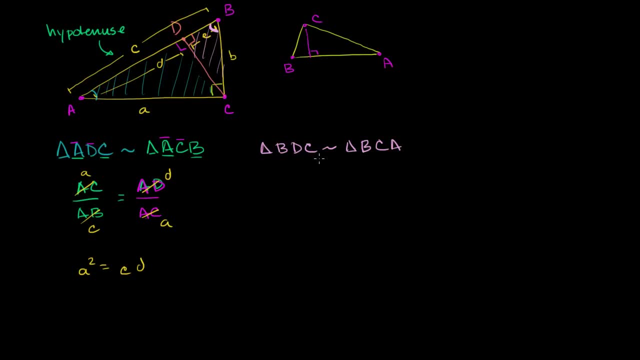 We labeled it before with that blue, So now let's set up some type of relationship here. We can say that the ratio on the smaller triangle bc side, bc over ba, bc over ba. Once again, we're taking the hypotenuses of both of them. 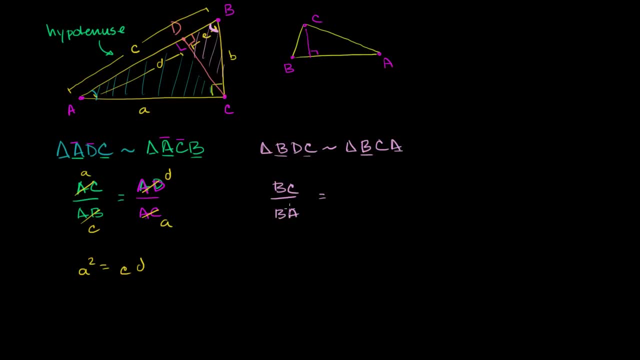 So bc over ba is going to be equal to bd. let me do this in another color bd. So this is one of the legs bd. The way I drew it is the shorter legs: bd over bc. I'm just taking the corresponding vertices. 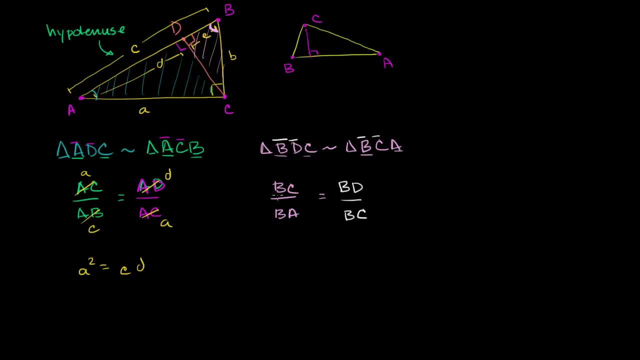 Over bc. And once again we know bc is the same thing as lowercase b, ba is lowercase c And then bd we defined as lowercase, So this is lowercase e. We can cross, multiply here and we get b times b, And I've mentioned this in many videos. 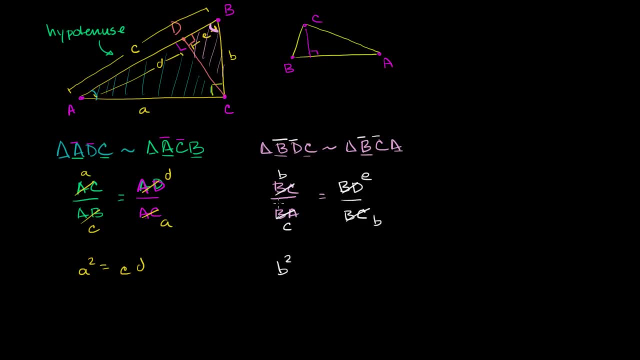 Cross multiplying is really the same thing as multiplying both sides by both denominators. b times b is b, squared is equal to ce. And now we can do something kind of interesting. We can add these two statements. Let me rewrite the statement down here. 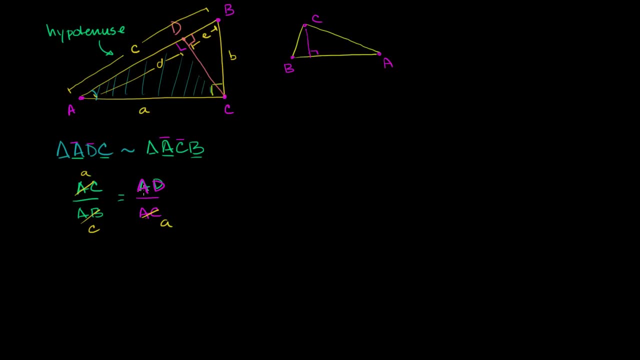 That'll just make things a little bit simpler for us. So AD we'll just call d, And so we have a over c is equal to d over a. If we cross multiply, you have a times a, which is a squared is equal to c, times d, which is cd. 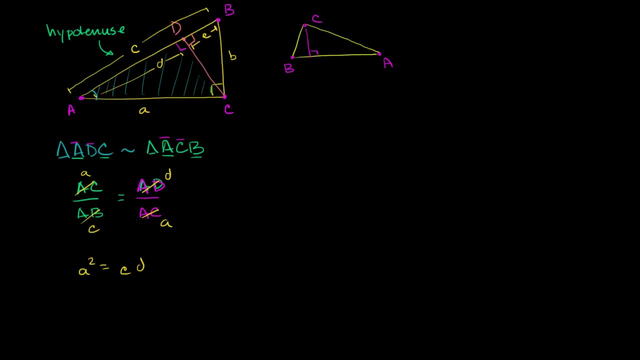 So that's a little bit of an interesting result. Let's see what we can do with the other triangle right over here. So this triangle right over here, So once again it has a right angle. The larger one has a right angle. 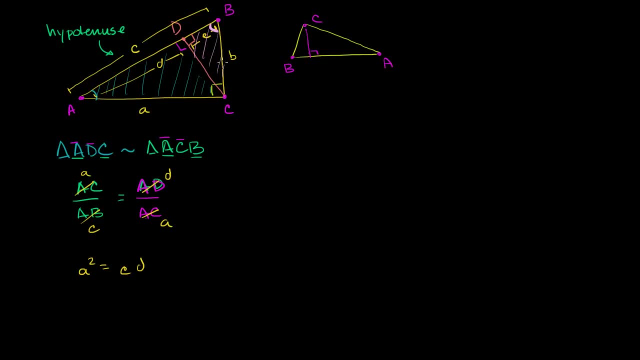 And they both share this angle right over here. So by angle-angle similarity the two triangles are going to be similar. So we could say triangle BDC. We went from pink to right to not labeled, So triangle BDC is similar to triangle. 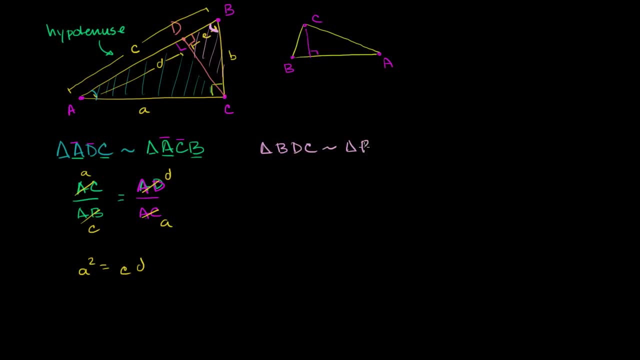 Now we're going to look at the larger triangle. We're going to start at the pink angle b Now. then we go to the right angle ca, From pink angle to right angle to non-labeled angle, at least from the point of view here. 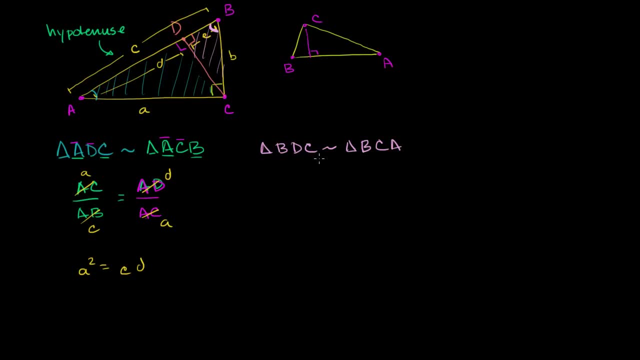 We labeled it before with that blue, So now let's set up some type of relationship here. We can say that the ratio on the smaller triangle bc side, bc over ba. once again we're taking the hypotenuses of both of them. 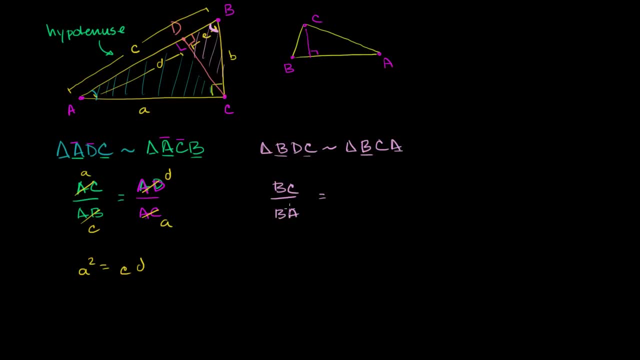 So bc over ba is going to be equal to bd. let me do this in another color bd. so this is one of the legs bd. the way I drew it is the shorter legs: bd over bc. I'm just taking the corresponding vertices. 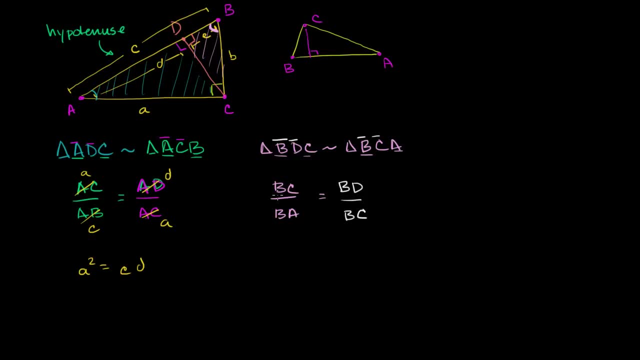 Over bc. And once again we know bc is the same thing as lowercase b, bc is lowercase b, ba is lowercase c And then bd we defined as lowercase, So this is lowercase e. We can cross multiply here And we get b times b. 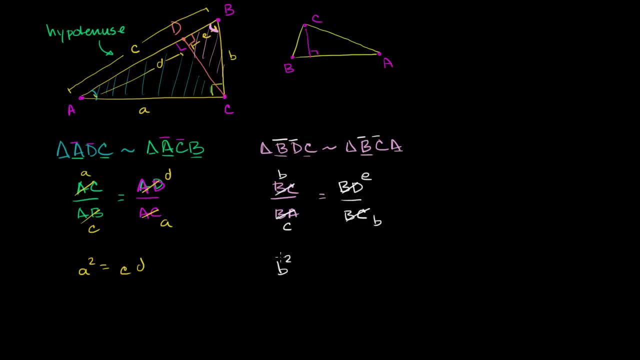 And I've mentioned this in many videos. Cross multiplying is really the same thing as multiplying both sides by both denominators. b times b is b, squared is equal to ce. And now we can do something kind of interesting. We can add these two statements: 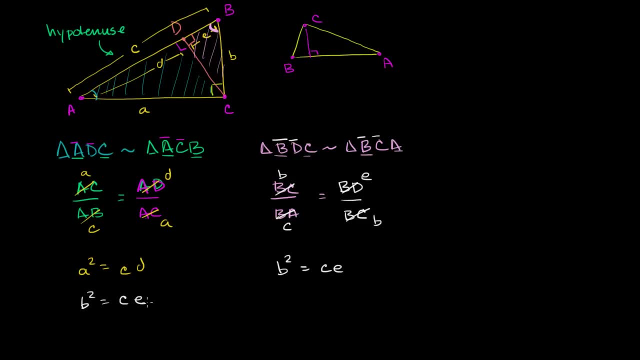 Let me rewrite the statement down here. So b squared is equal to ce. So if we add the left-hand sides, We get a squared plus b squared is equal to cd plus ce, And then we have a- c in both of these terms. 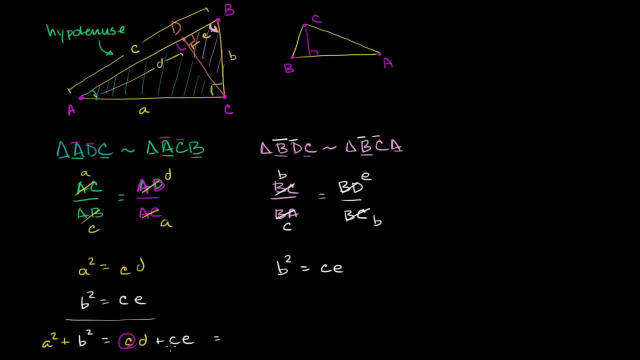 So we could factor it out. So this is going to be equal to. We can factor out this: c. It's going to be equal to c times d plus e. Close the parentheses. Now what is d plus e? d is this length. 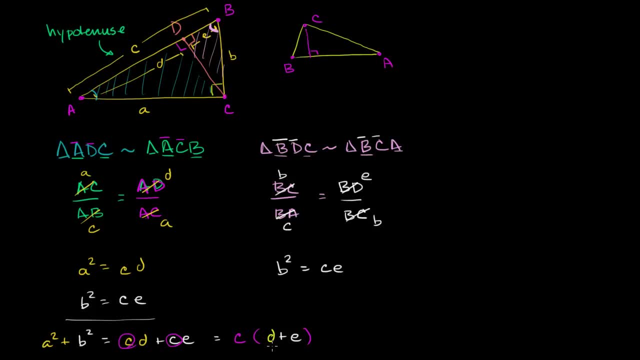 e is this length, So d plus e is actually going to be c as well, So this is going to be c. So you have c times c, which is just the same thing as c squared. So now we have an interesting relationship. 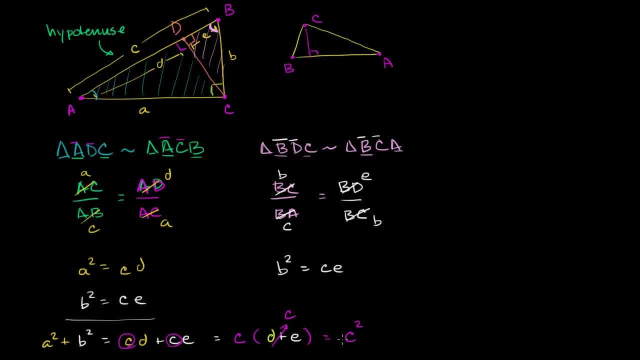 We have that a squared plus b squared is equal to c squared. Let me rewrite that a squared. I'll do that. Well, let me, just in an arbitrary new color. Actually, let me. I deleted that by accident, So let me rewrite it. 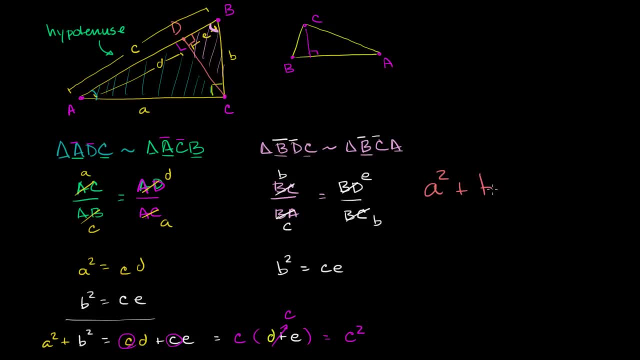 So we've just established that a squared plus b squared is equal to c squared, And this was just an arbitrary right triangle. This is true for any two right triangles. We've just established that the sum of the squares of each of the legs is equal to the square of the hypotenuse. 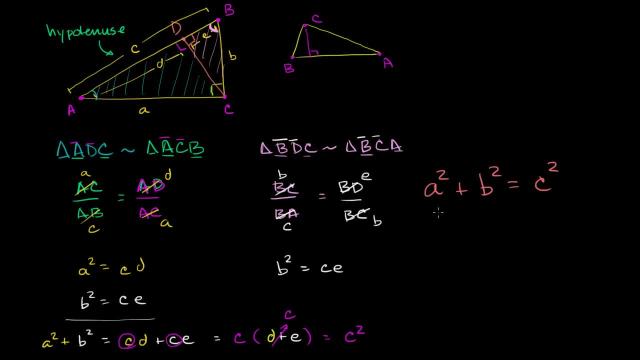 And this is probably one of the- well, it's easily one of the most famous theorems in mathematics, named for Pythagoras. Not clear, He's the first person to establish this, But it's called the Pythagorean theorem. 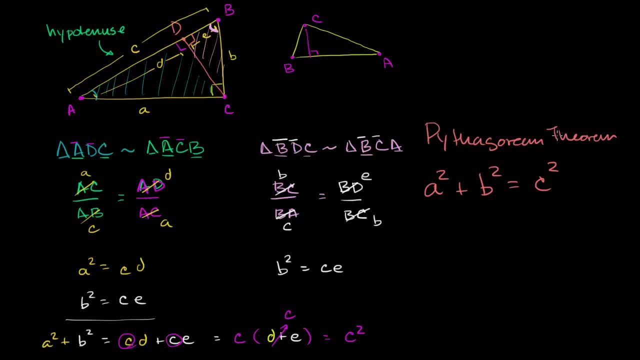 And it's really the basis of- well, not all of geometry, but a lot of the geometry that we're going to do, And it forms the basis of a lot of the trigonometry we're going to do, And it's a really useful way. 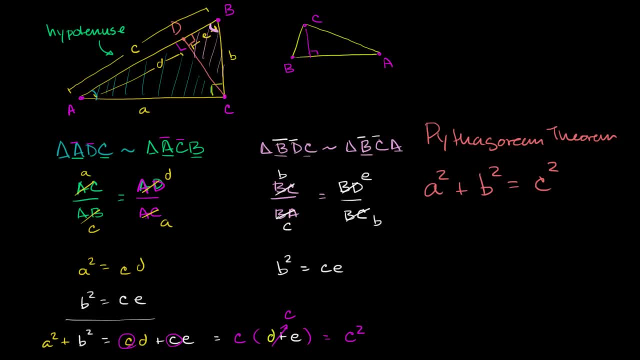 If you know two of the sides of a right triangle, you can always find the third.